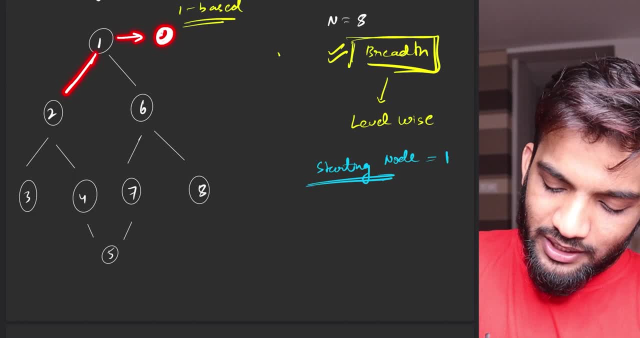 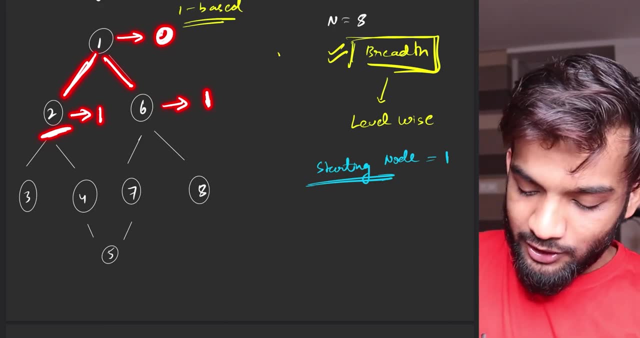 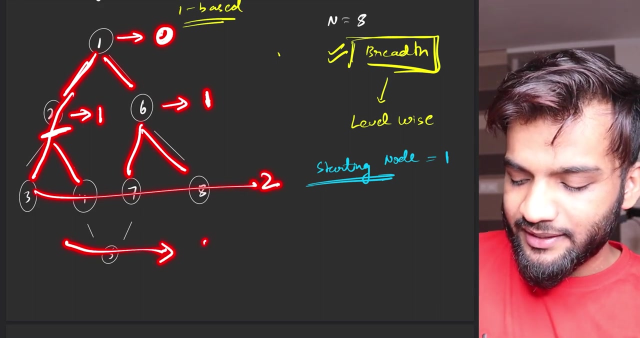 generally say this is at level zero, and then you say this: these guys are at a distance of one, so you'll call them as level one. then you say these guys are at level two and then you see this guy is at level three. so what you do is, in breadth first search traversal. 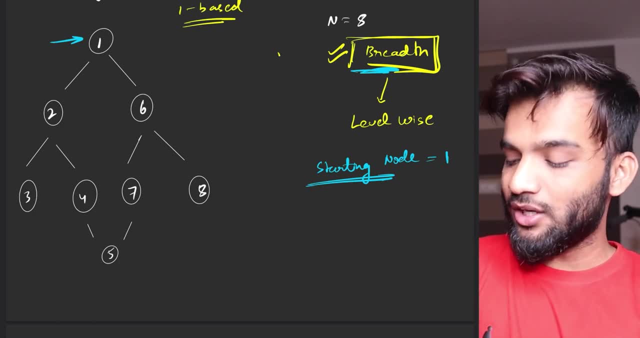 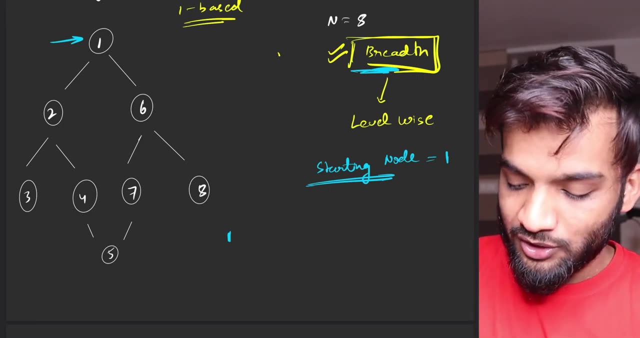 first you visit the first cat. that is the starting node and you write that so that that is something that you have written. then you go to all the guys that on the next level. so this was at the zeroth level, so the next level will be nothing but first. so i can say this: 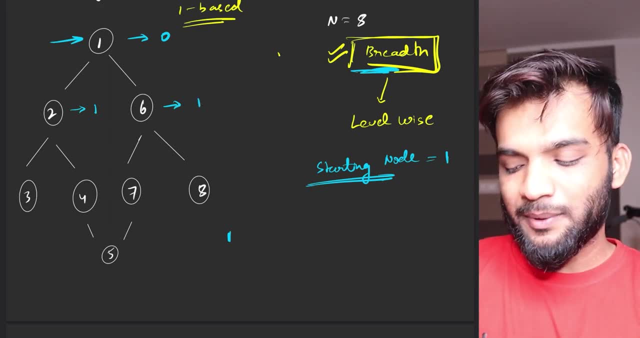 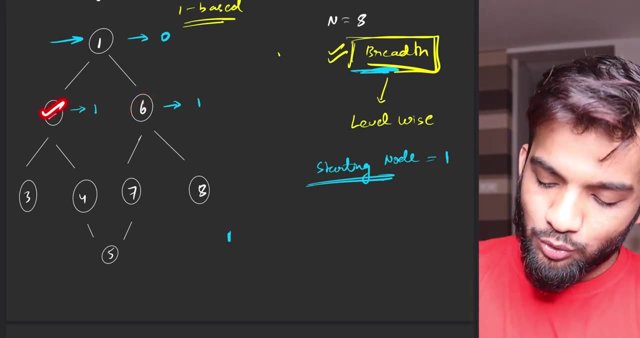 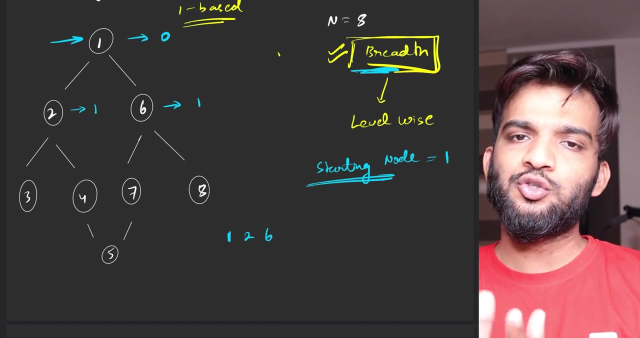 is at the first level. and this is at the first level. now, in the breadth, first breadth, first search traversal, you can either traverse this and then this, or you can either traverse two and then six. that is completely your choice. so I will decide to travel to six. you can travel six to as well, that is completely okay. so this: 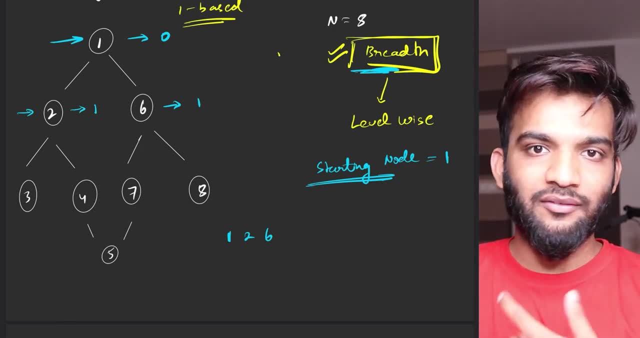 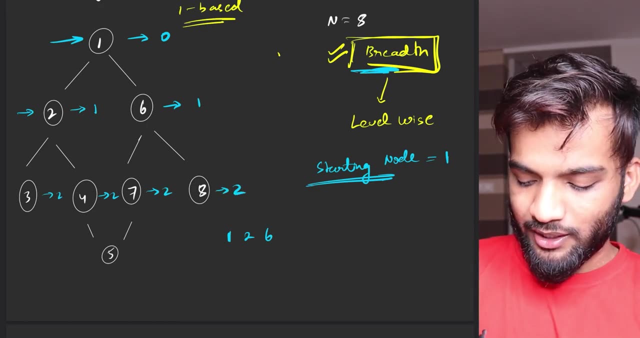 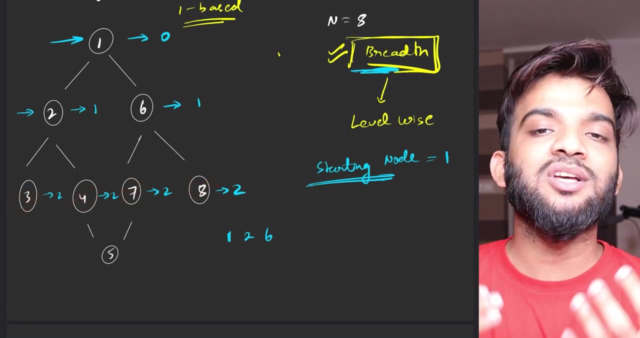 is also done. now the next level is level two and you know these all guys are level two, correct? so what do you do? is you say, okay, again, you can write three, four, seven, eight. you can write something like eight, seven, four, three. that is completely your choice, as long as you are traversing all the nodes in 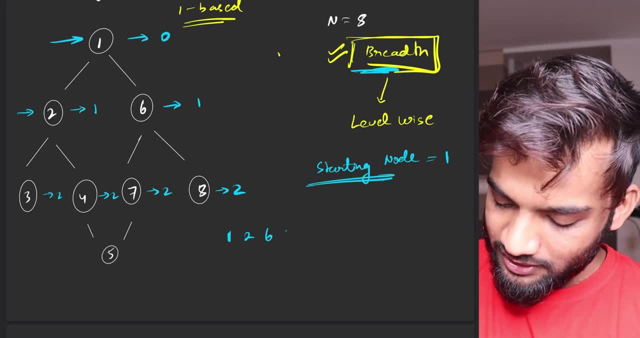 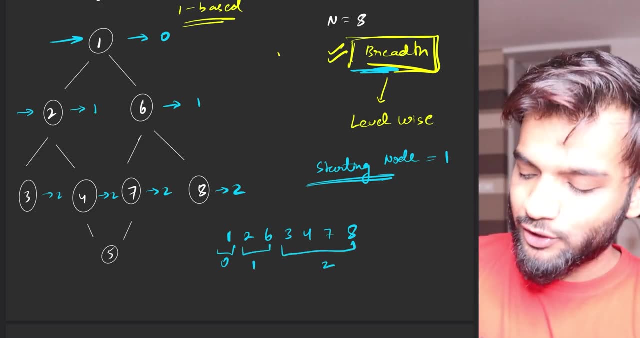 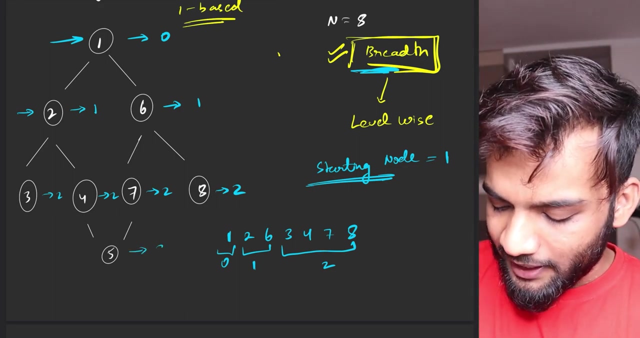 the level wise fashion. we are completely okay with it. so it is like three, four, seven, eight. so see, this is level zero, this is level one and all of these are level two. so the level two can be traversed in any of the ways, but they should be travel together, okay. next will be level three, and this is level three. 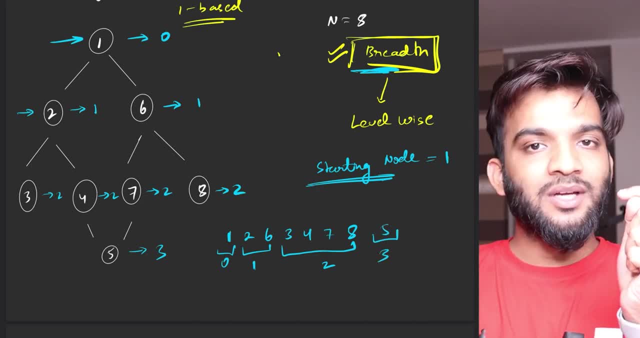 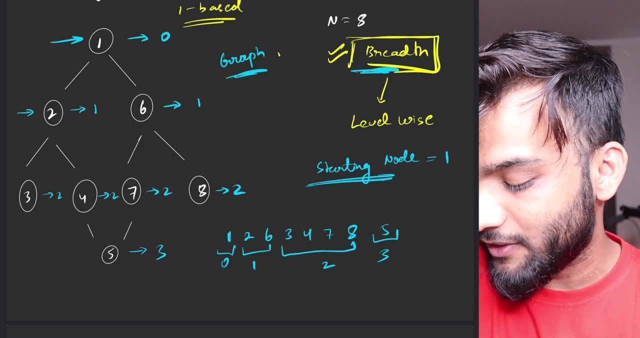 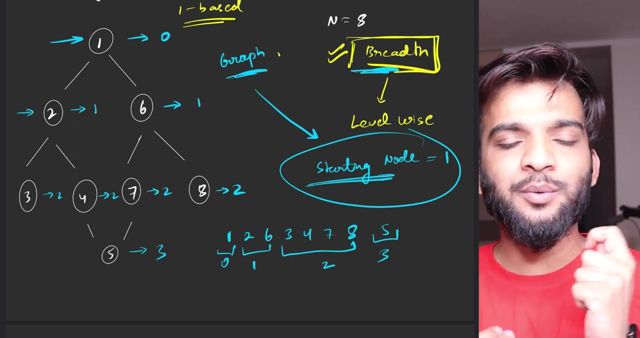 so I can say this is level three. so this will be the breadth first BFS traversal of this particular graph. but if the starting node is one, very, very important, if the starting node is one, what if I change the starting node? so let's quickly change the starting node. 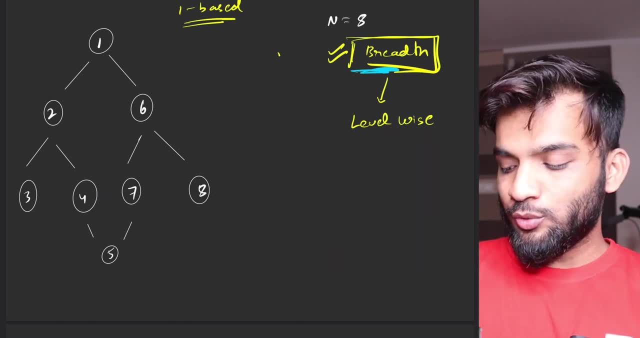 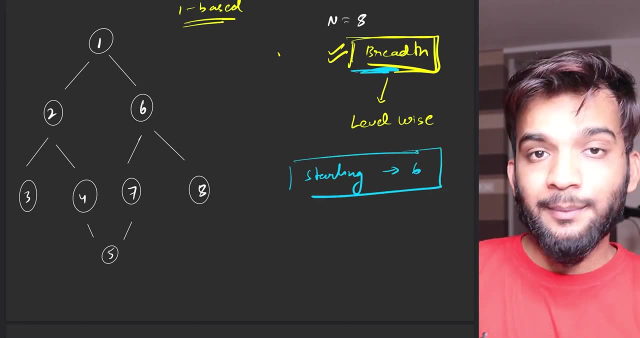 and understand BFS in depth. so, as you, I tell you that the starting node as of now is six. okay, so I've changed the starting node. remember this: this is the starting node, and this is the starting node, and this is the starting node and this is at level zero. if this is at level zero, you cannot say this to be at. 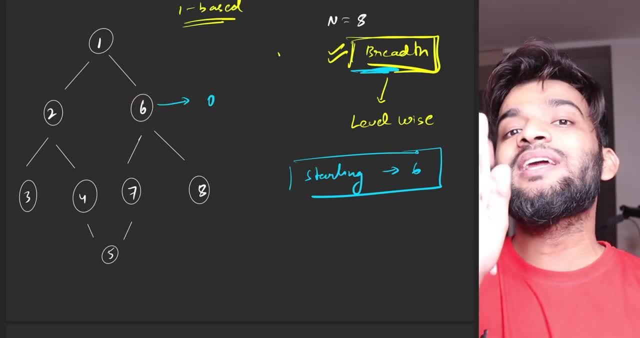 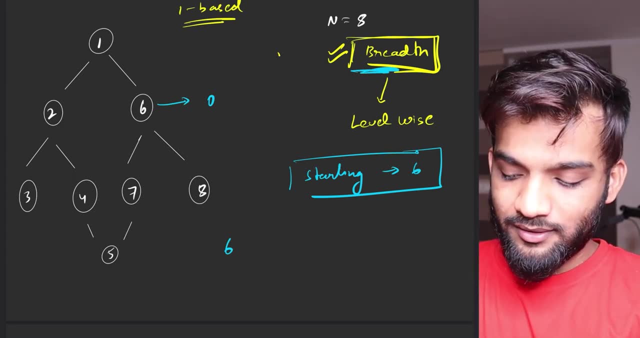 level zero. no, this, only one node can be at level zero. so you write six at level zero. if I ask you which it which is at level one, then what do you do? is you say: this is at a distance one, this is at a distance one, this is at a distance one. 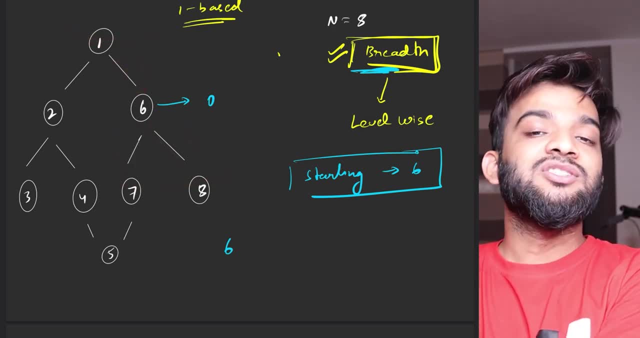 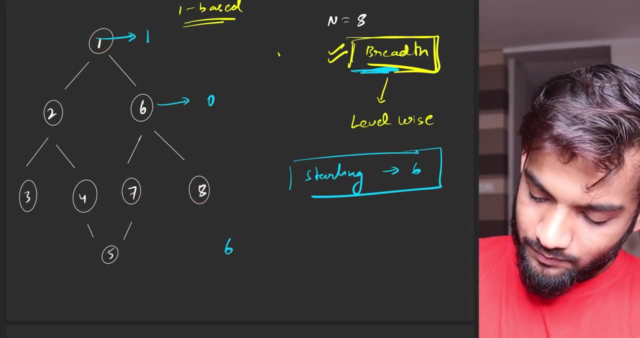 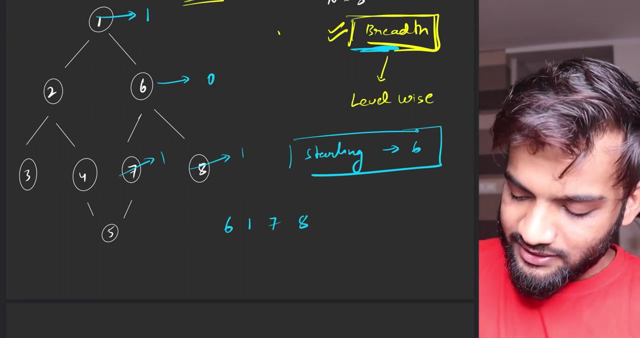 so all of these guys are at equivalent distance. very, very important. all of these guys are at equivalent distance, so thereby you call them as level one, level one and level one again. you can travel one first, then seven, then eight. that is your choice. so I'll decide to travel one, seven, eight. so this is level. 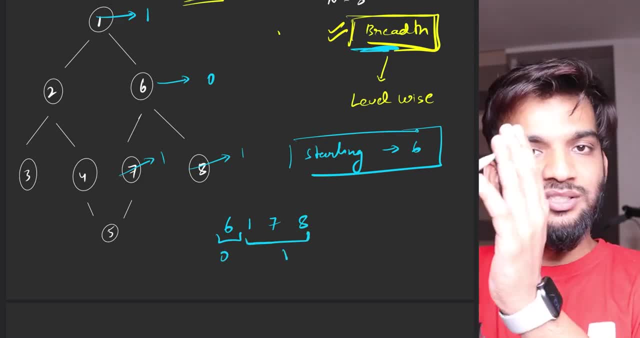 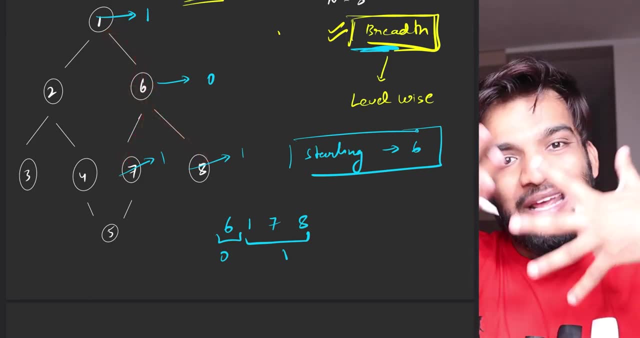 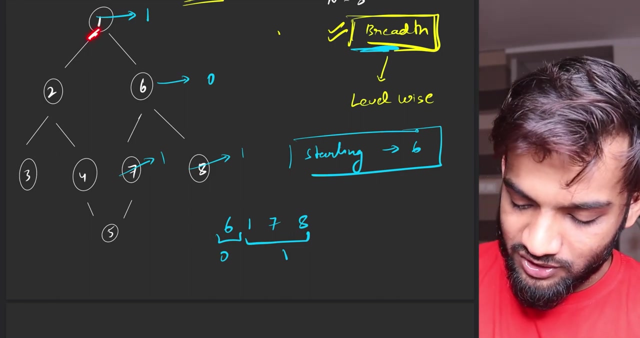 zero. this is level one. you need to understand the distance. distance breadth. it goes equal in the breadth. so it was here, it went equivalent in the breadth. that is very important to understand. okay, wwwbfssnetinslu ask you. the next level, that's two. so for this, this is level two. this is level two. and are there? 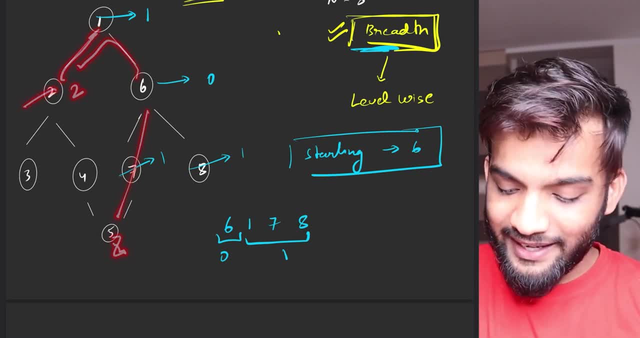 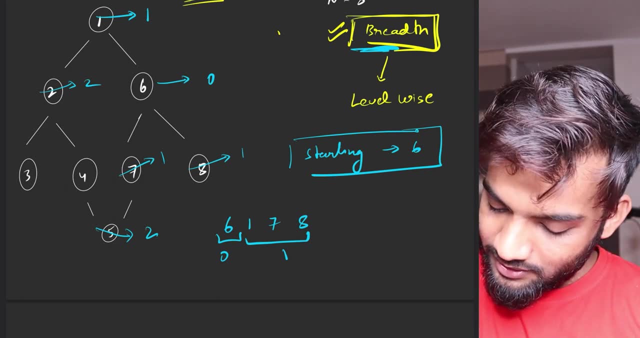 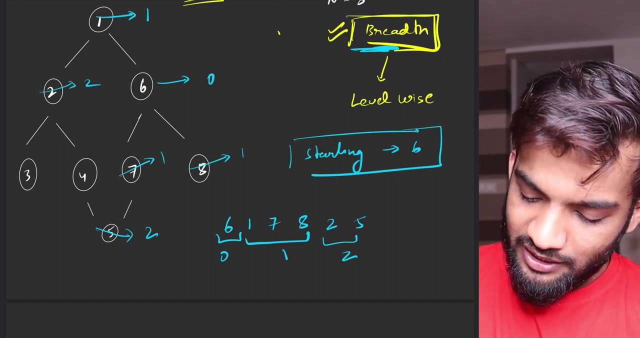 anyone else who is level two. i don't see. so i can say, okay, this guy is level two and this particular guy is level two. so you can again write something like two and five. so this is level two, perfect, and it's time for level three. so obviously, one, two, three. so this will be three. so maybe one, two. 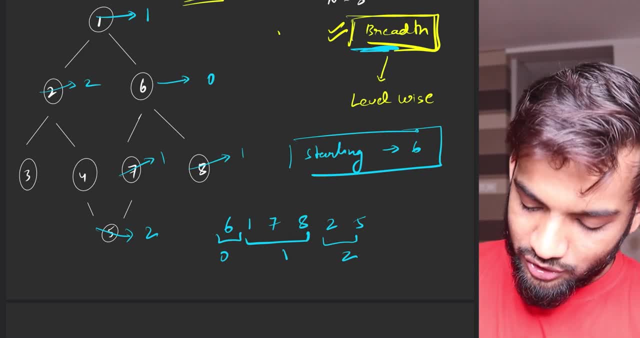 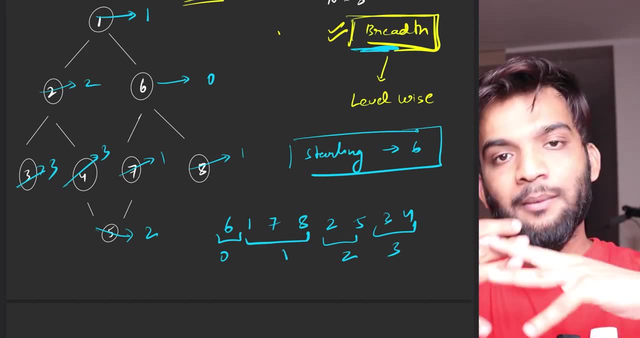 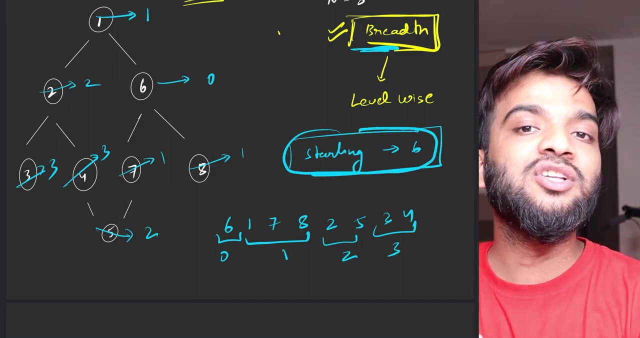 three, this will be three. and are there any other? no, so this is three, this is three. so there are two guys who are three. that's very important. you travel breath wise, breath wise, and everything depends on the starting node. depending on the starting node, the traversal will change and you. 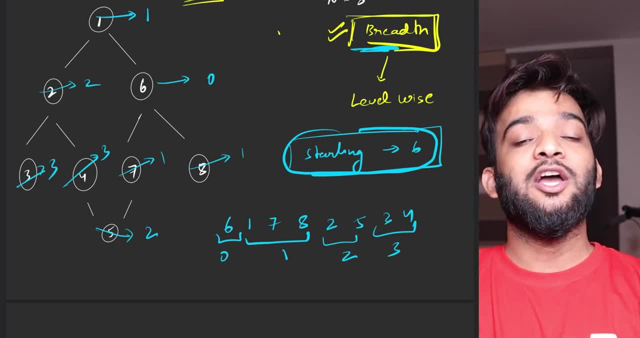 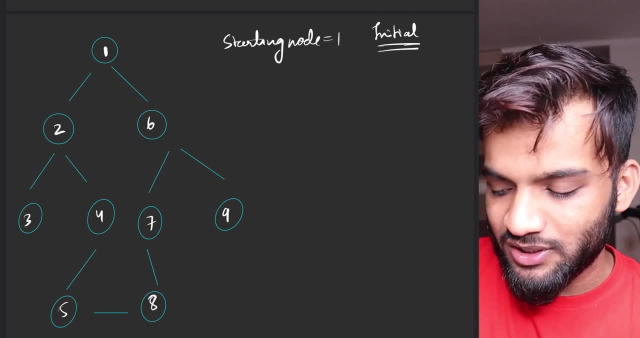 will always travel in the breath wise manner, in the breath wise manner. i hope that is clear. in order to do a bfs traversal, there is an initial configuration that you need to start off with. so, whatever is the starting node given to you, what you do is you clearly take a queue data. 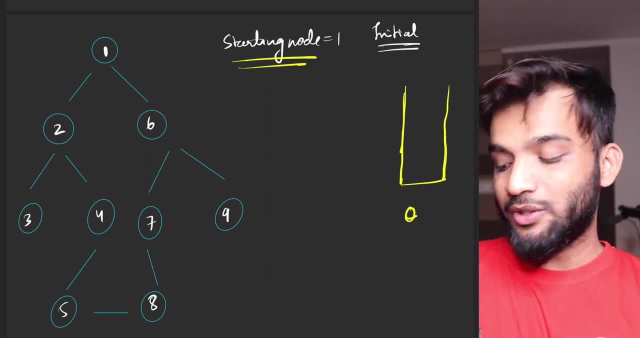 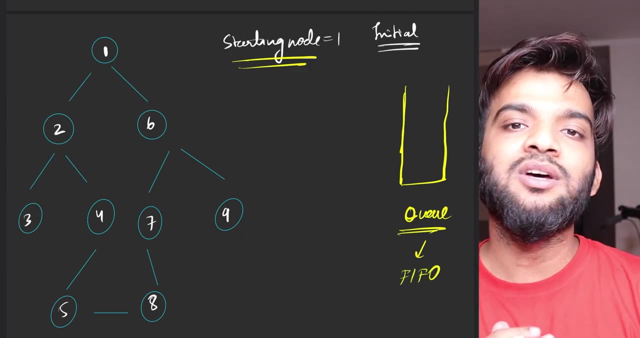 structure. now, if you don't know queue data structure, please read about that. you take a queue data structure. queue is nothing but first in, first out. the guy who goes in first gets out first. so the initial configuration says i am going to define a queue data structure and that will. 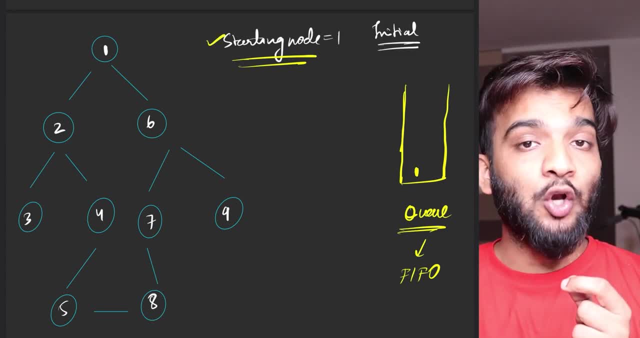 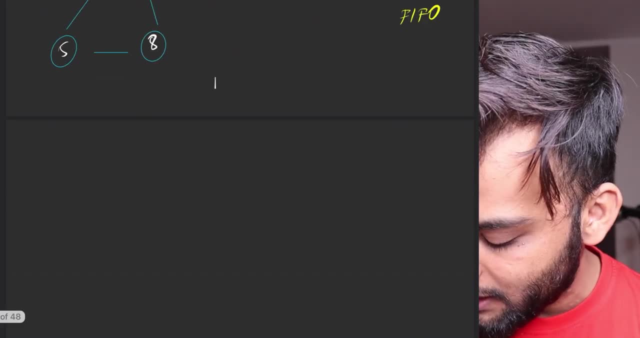 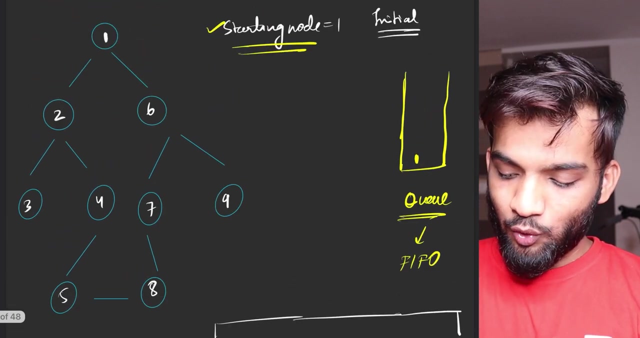 always contain this particular guy. remember this. that will always contain this particular guy, starting node. and there is another thing that you need to do. you need to create something as a visited array, okay, and this visited array is something which is very common in all the graph questions and over here, if you. 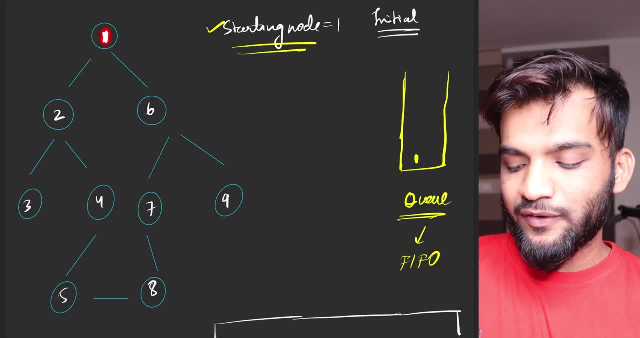 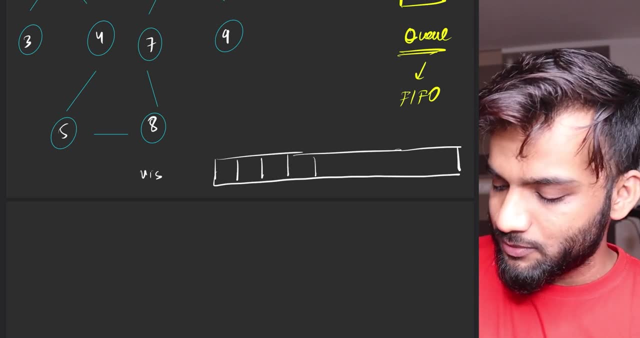 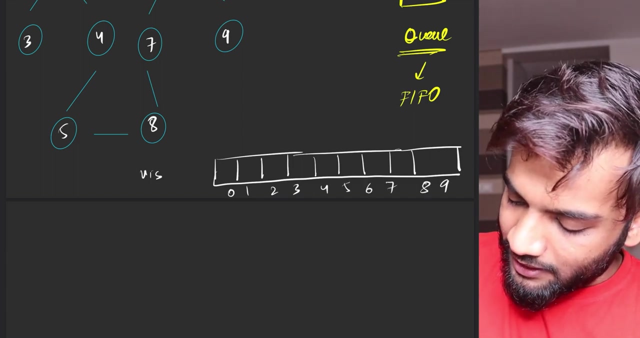 see, the node is numbered till nine and since the graph is one based, what you'll do is you'll create this visited of a size 10. okay, please make sure you create of a size 10. so this is like zero: one, two, three, four, five, six, seven, eight, nine, so this will be the visited one. 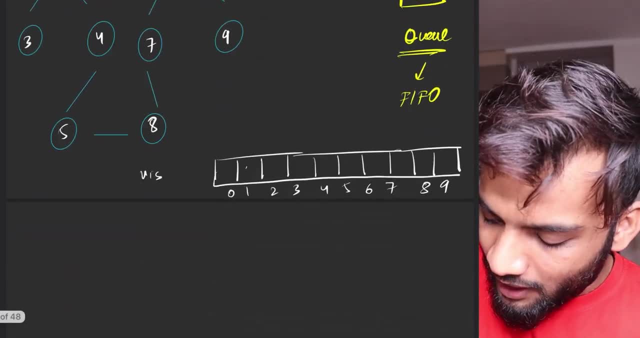 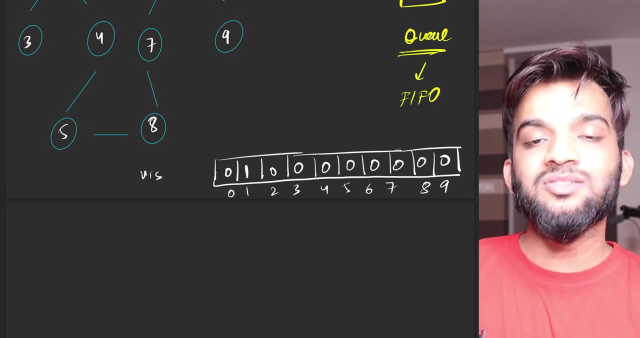 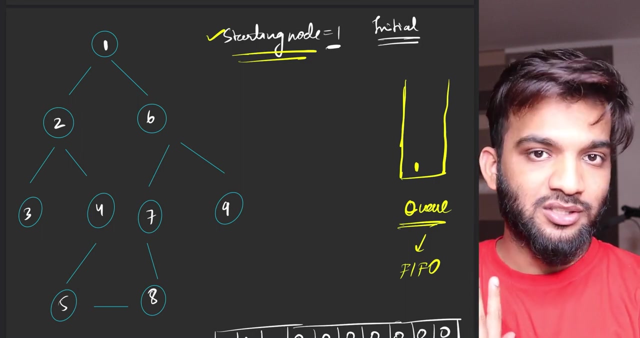 and whatever is the starting node, you go over there and you mark it as one and everyone else will be marked as zero. so over here, please understand this one means this guy is already in the queue. whenever i say someone has been traversed, someone has been touched, wait, mark that as visited. this will be the initial 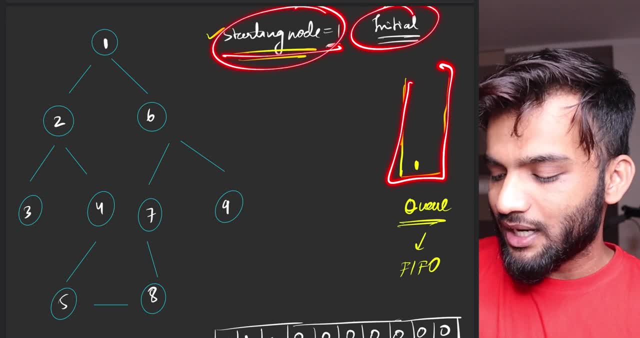 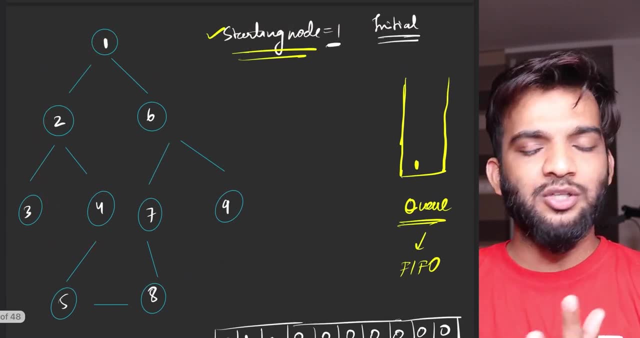 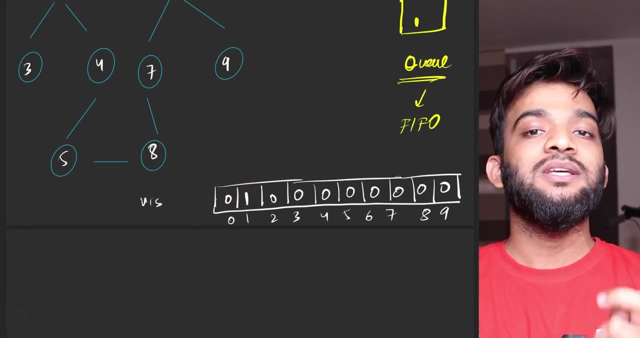 configuration: initially a queue which contains a starting node. initially a visited array which will be of size depending on its one. based or zero based, you can decide- and the starting node will be traversed, so thereby it will be marked as one. this is going to be the initial or the starting. 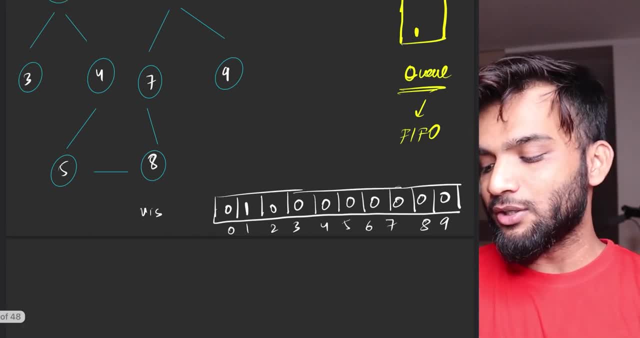 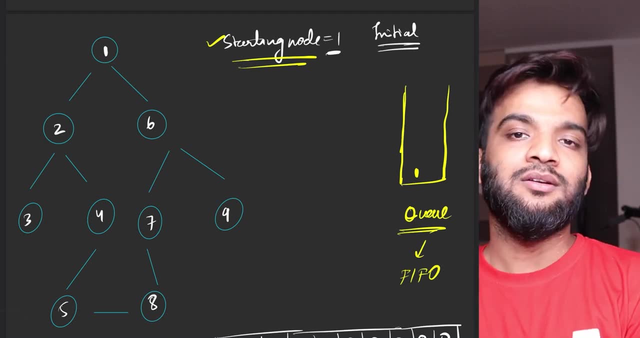 configuration in a bfs traversal. what is the next step that you will do? whatever is in the queue, you will start taking it out. start taking it out. start taking it out till the queue is not empty. remember this: keep taking out. keep taking out till the queue is not empty. 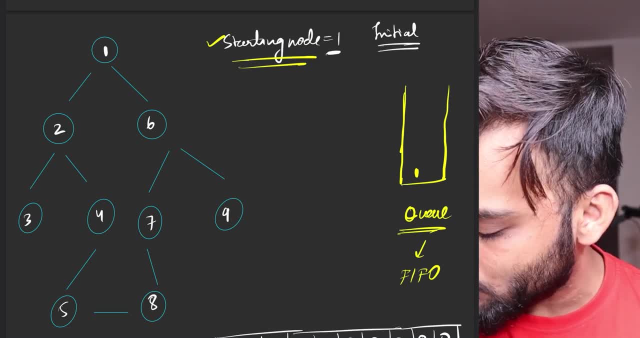 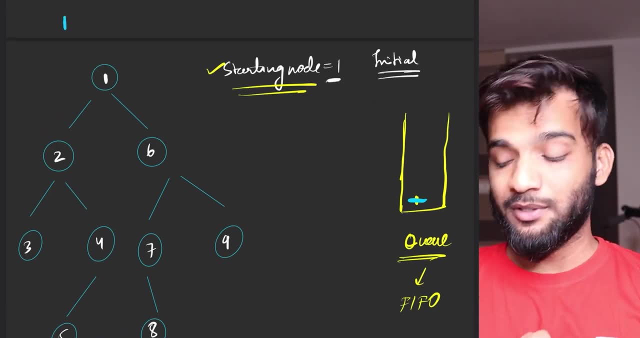 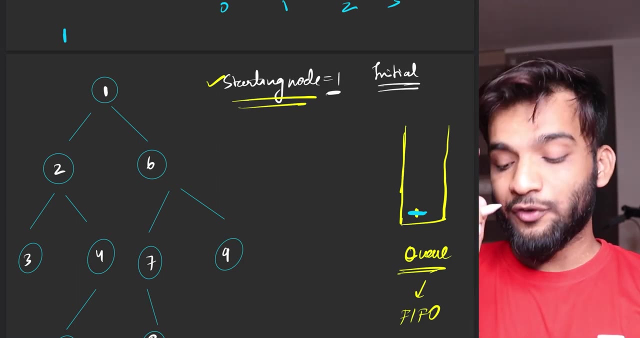 okay, so whatever is it the uh q data structure, i take it out and you'll print it. so assume i print this. so this is printed. right, this is printed as a bfs travesty. now, very important. whatever you take out of the queue, one you took out of the queue, so if you remember this graph. 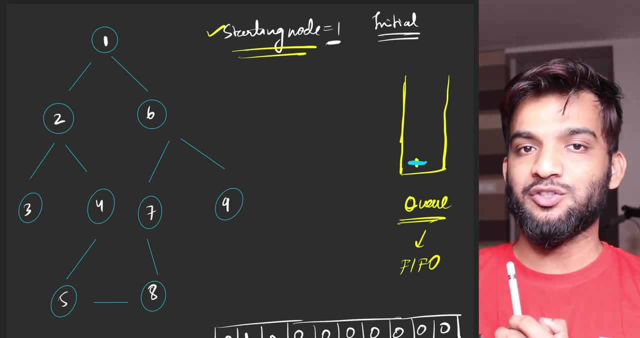 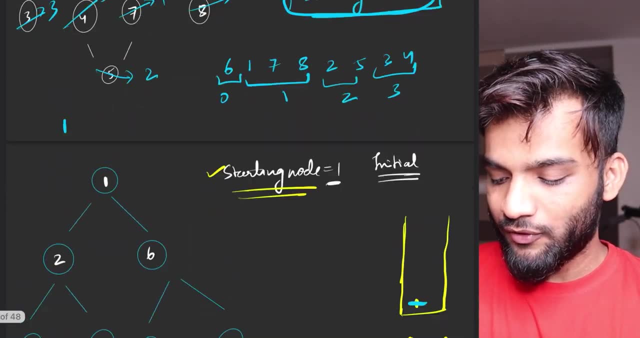 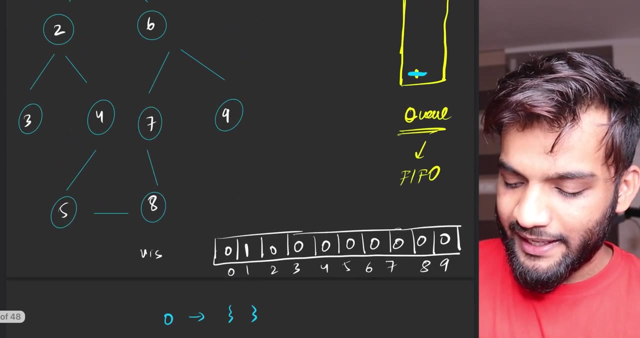 you would have stored this in some data structure, and which data structure was that? that data structure was adjacency list, do you remember? yes, so what will be the adjacency list for this particular graph? can i say? for zero, it will be an empty data structure. for one, it will be storing this. two and six, remember this. 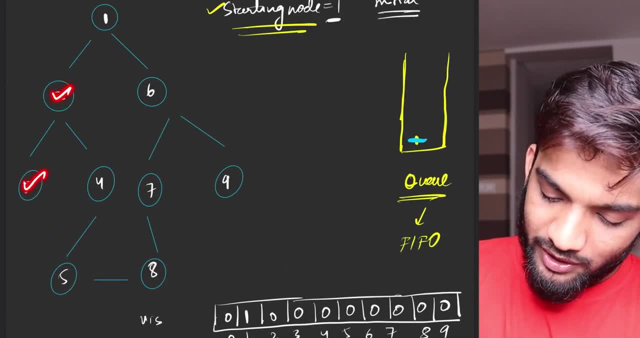 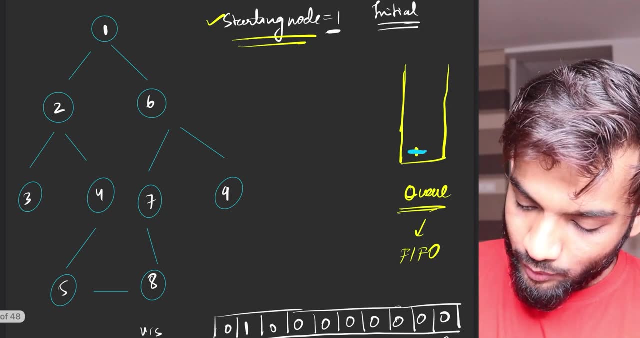 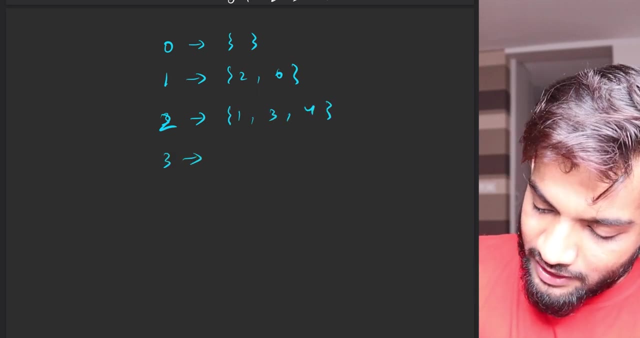 okay, let's write for the next for three. it will just be storing two, so please write that. sorry for two. you have to write in the next step for two. it will be storing one, three and four, so let's write one, three and four. next will be for three. let's check out for. 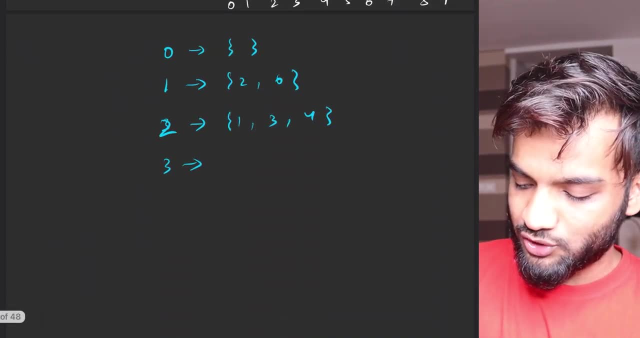 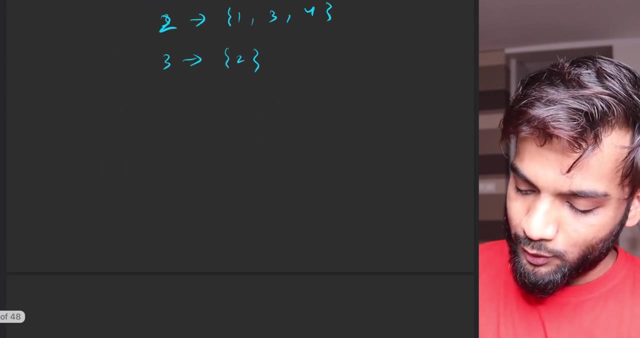 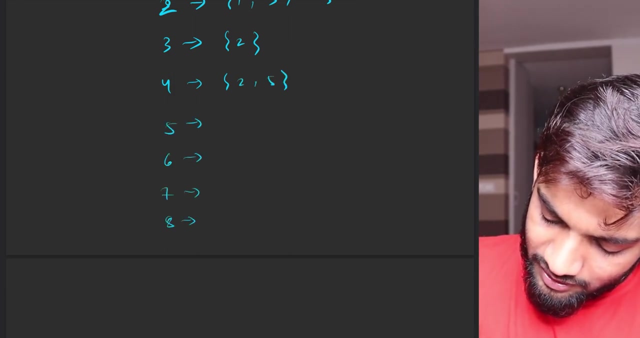 three for three. it's just storing two, so let's uh store two in it. next will be four for four. it is having five and two, so for four it will be two and five for five, for six, for seven, for eight, similarly create the entire adjacency list. 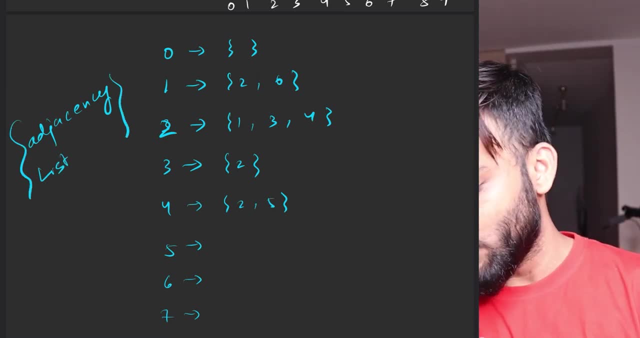 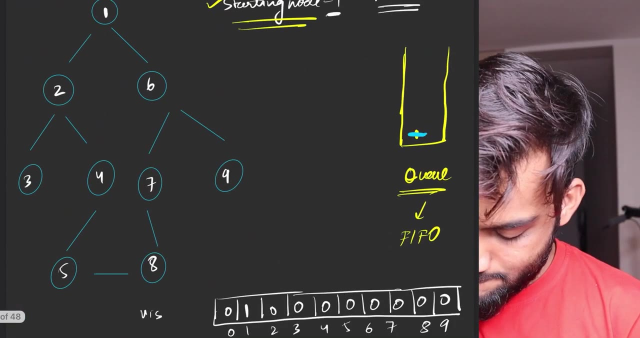 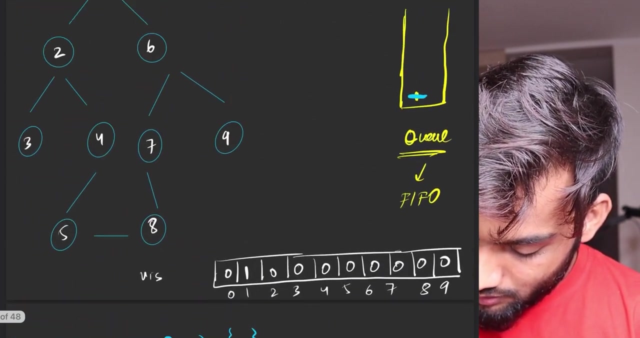 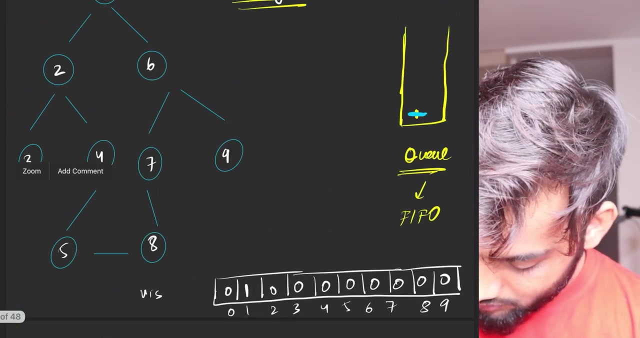 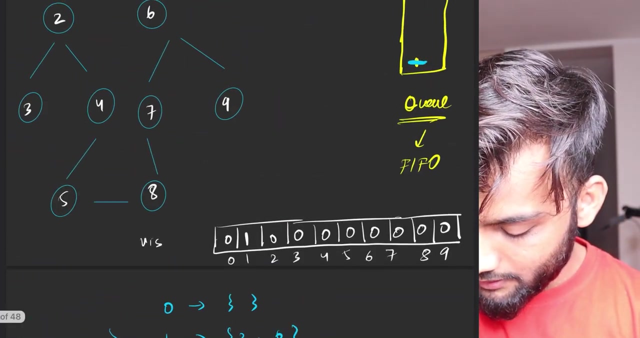 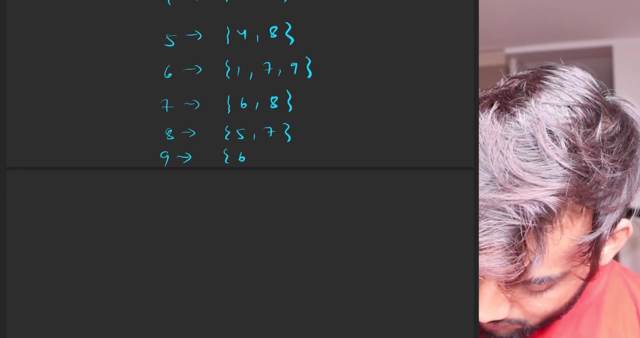 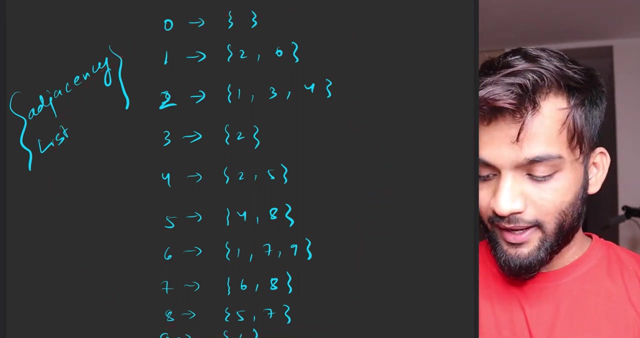 that i have already taught you in the second video. so kindly create this, and after that we can start off with the bfs traversal. this is good, okay, so. so this is how the entire adjacency list will look like now. whenever you take the first element out and you print it, what you do is: 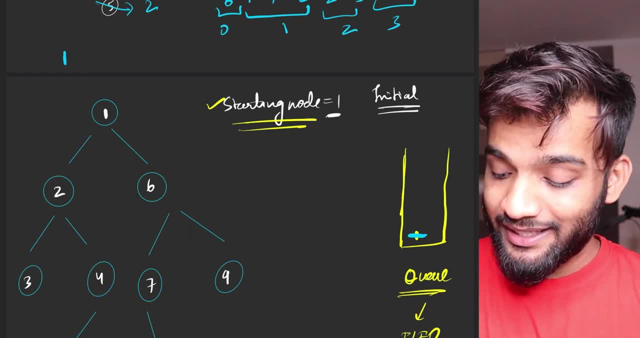 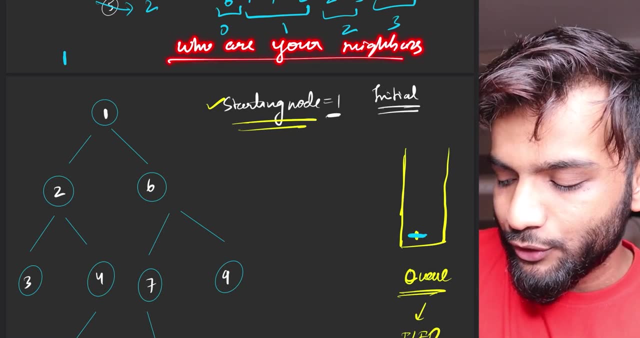 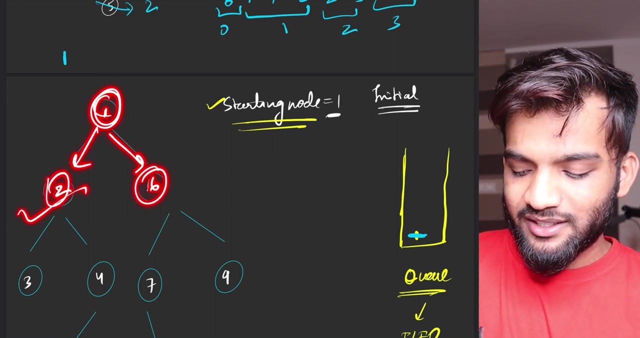 you go to one and you say: who are your neighbors? i, i repeat, you ask: who are your neighbors? okay, and how will you know who are its neighbors? if you remember well enough, in the graph, you can see that two and six are its neighbors. two and six are its neighbors who are at an equivalent. 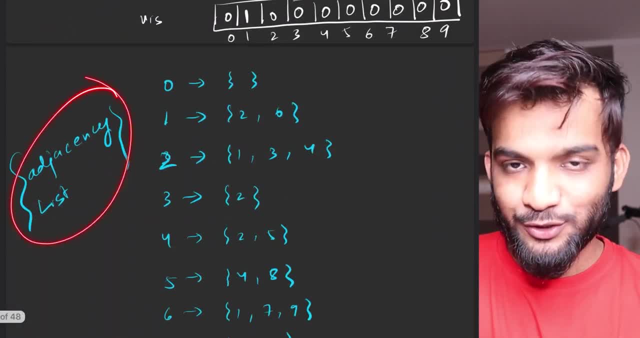 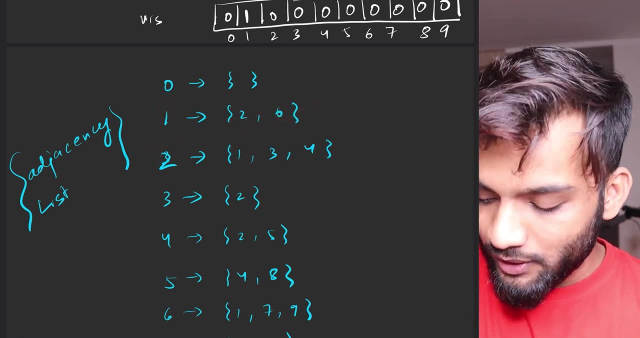 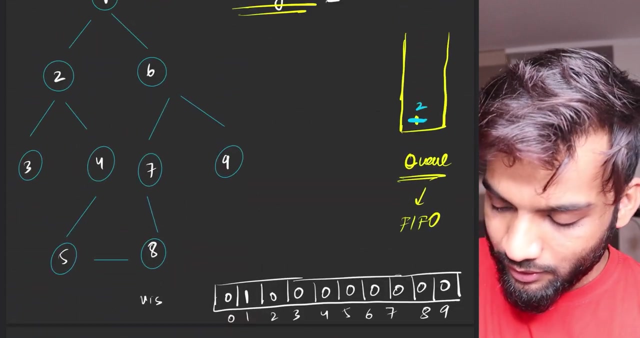 distance. so if you remember, this guy stores all the neighbors- remember in the second lecture i told you so- who are the neighbors of one, two and six. so what you do is you take two, you take six. first take two, put that into the queue data structure, okay, and mark it as one, next take six. 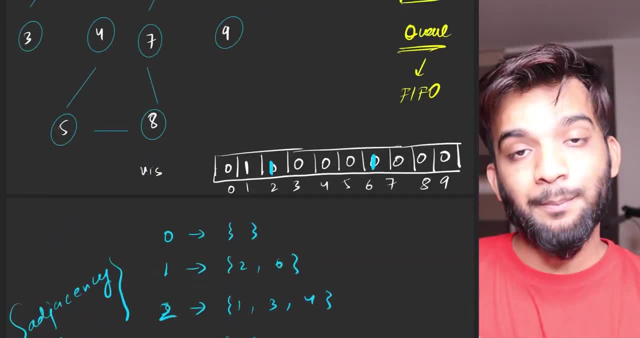 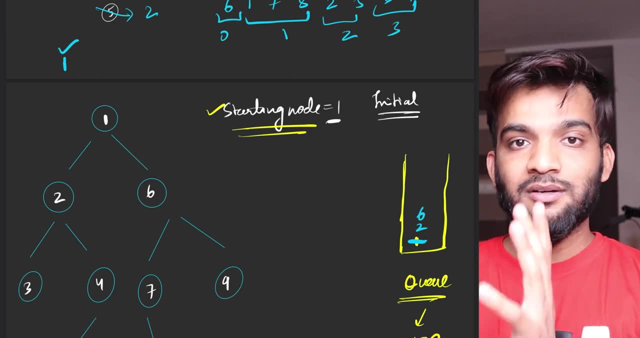 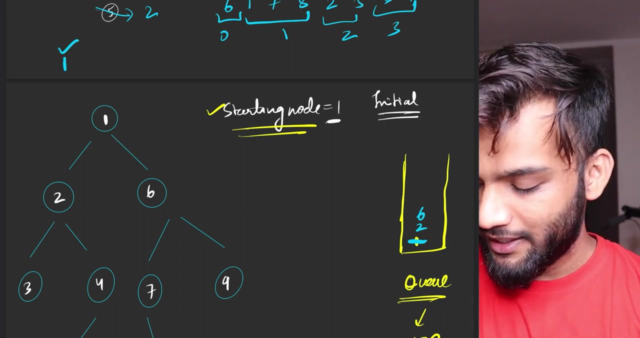 put it into the queue data structure and mark it as one. perfect done so. first, iteration of one is done, so it is very simple. let me repeat: you took out one. you basically went to its neighbors and you put that into the queue and marked it as visited. next time, take out the next guy, so i'll. 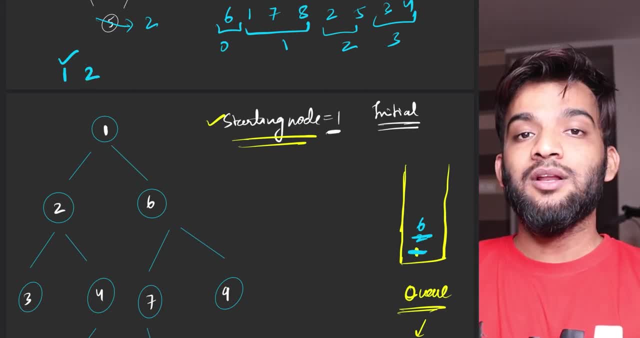 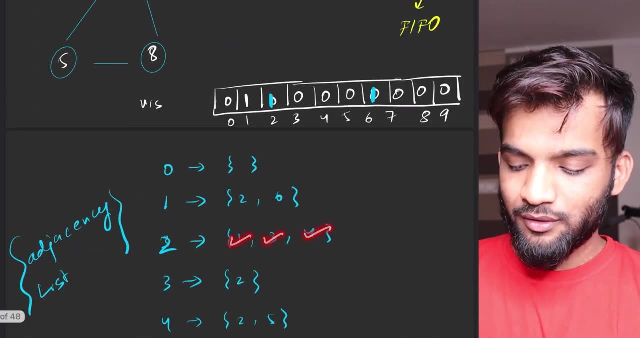 take out the next guy too. do the same thing again. take out the next guy and mark it as one same thing on this two as well. go to two's neighbors who are two's neighbors. how will you know again, two's neighbors are one, three, four. very obvious: one, three, four are its neighbors and that. 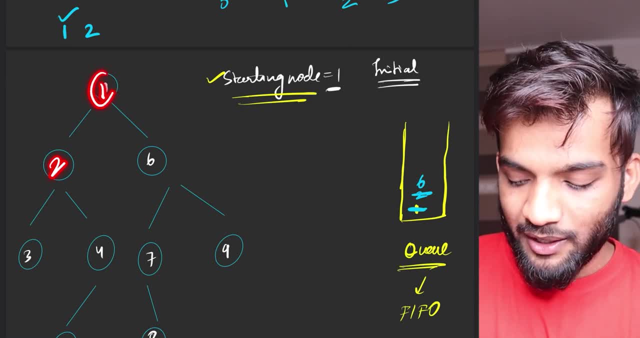 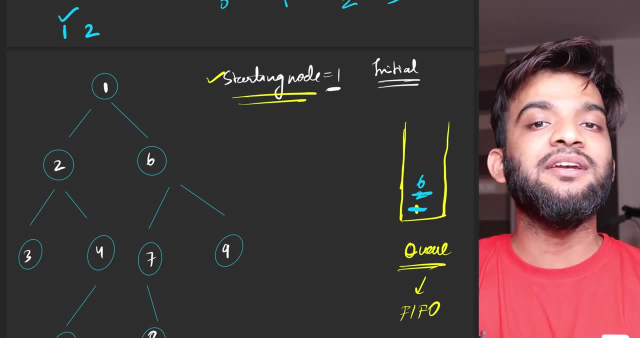 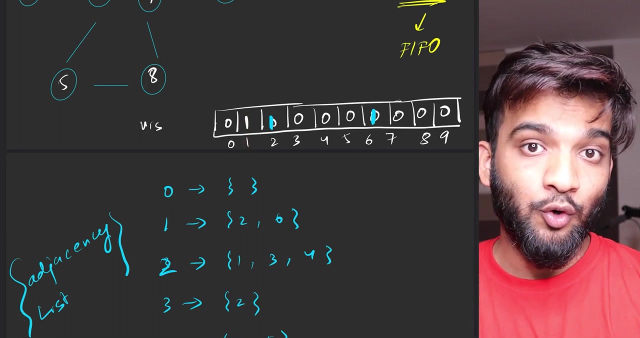 is stored in the adjacency list, so two's neighbors were one. but remember, this one will not be put into the queue. why? because you've already traversed one, because you've already traversed one. how will you know that? because, because, yes, one is already marked as visited, so you already know one. 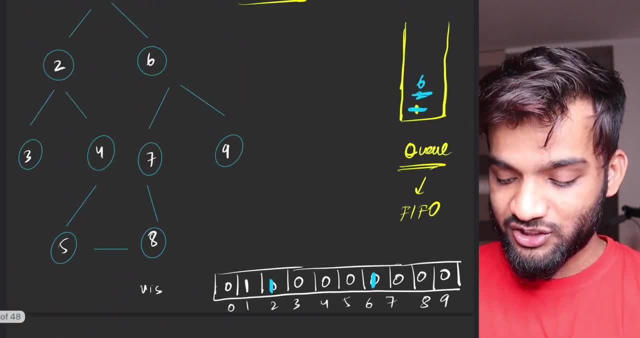 has to be put into the queue, so you already know one has to be put into the queue, so you already know one has been touched or traversed, so you'll not take one. instead of that, what you'll do is you will simply, uh, omit one and you'll not put that into the queue. let's check out the next. 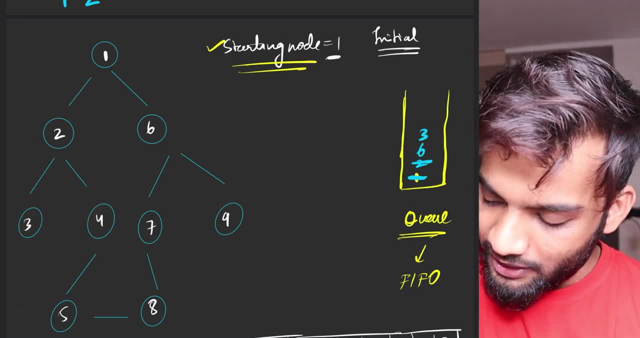 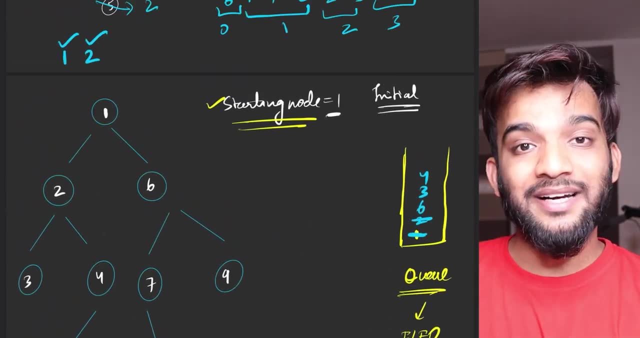 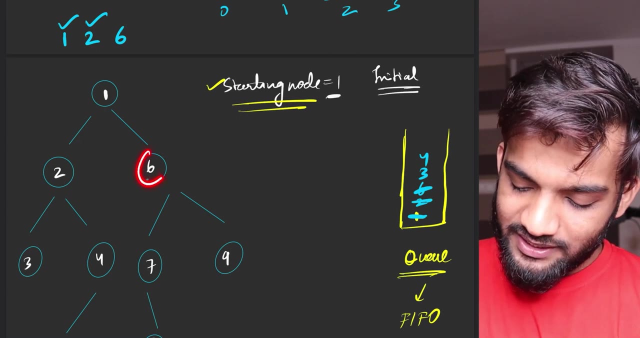 it is three and four. so you'll just take three and you'll take four and put that into the queue and mark three and four as visited. perfect, this is done. next you take the next element out: six. so six is there again. do the same thing for six, who are six? neighbor one already visited. 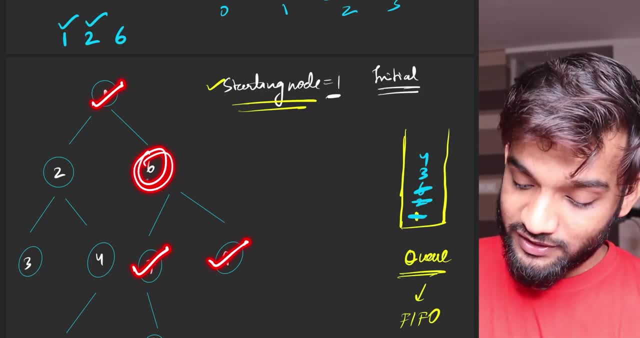 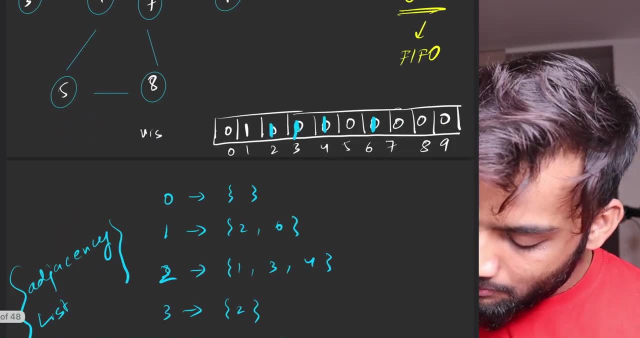 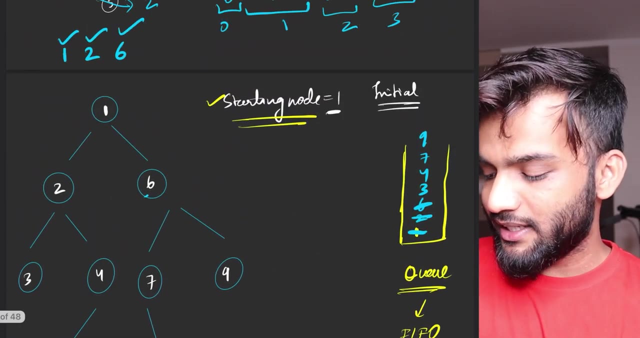 seven, not visited, nine, not visited. so you take seven and you take nine and you put that into the queue data structure at the same time. mark seven as true, nine as true, perfect, done. six is done. what's the next thing? three: let's take out three who are three's neighbors. just two already. 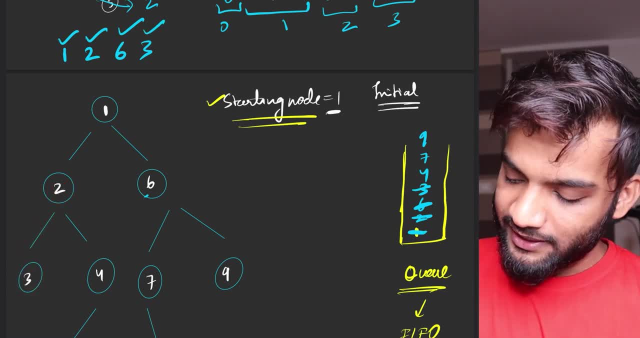 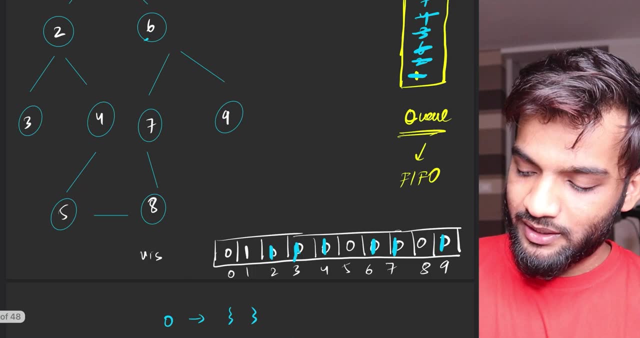 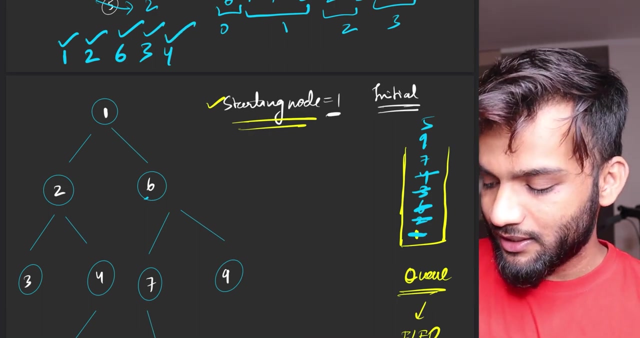 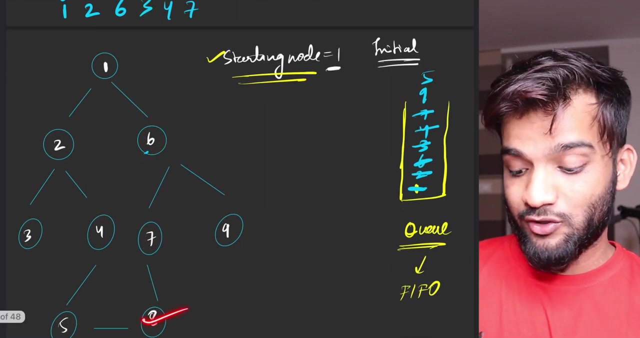 visited nothing to do so. three is also done. let's take the next one out. four, who are four? neighbor two already visited five. take five. put that into the queue. mark five as true perfect. four is also done. next, take seven, who are seven neighbors. six visited, eight not visited: take eight. 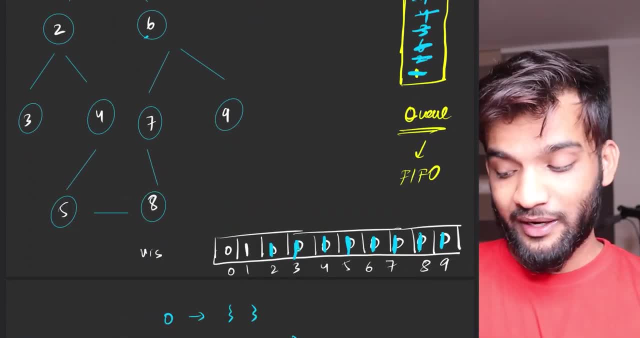 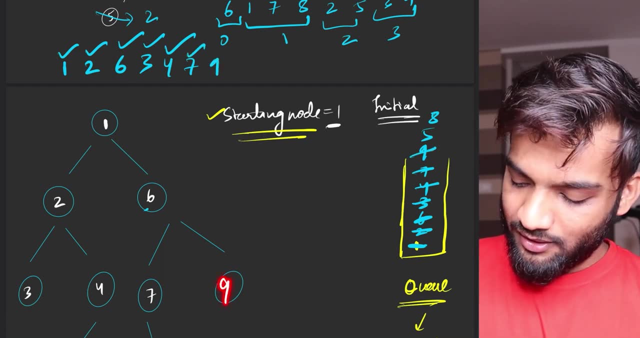 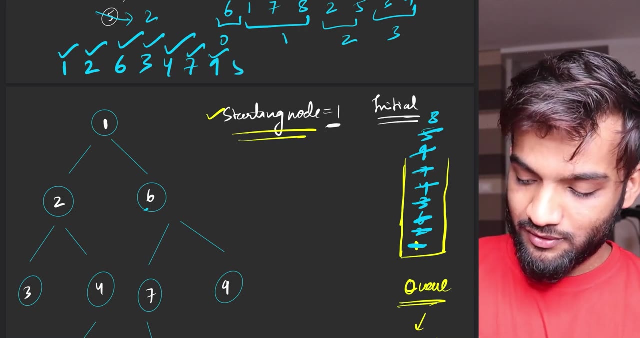 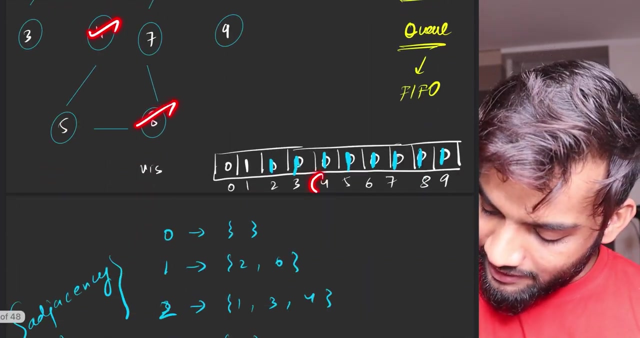 and put that into the queue and mark it as visited. perfect. next, so nine, what? what about nine for nine? there's one neighbor six, but that is already visited, so done. next, take five for five. who's the neighbor four and eight. and if you carefully see, four and eight are already visited. 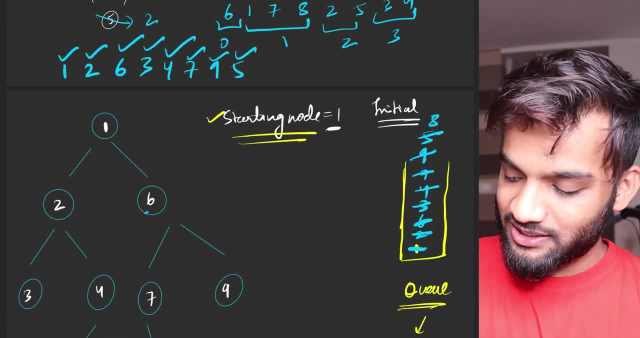 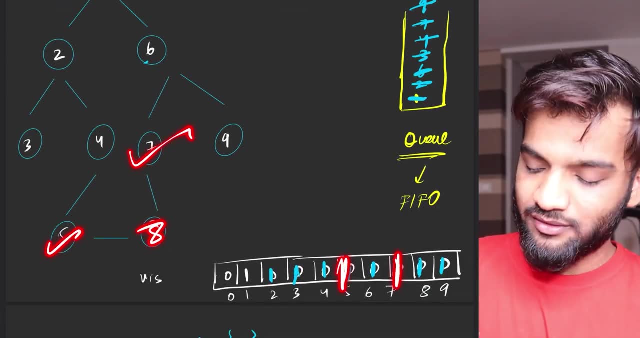 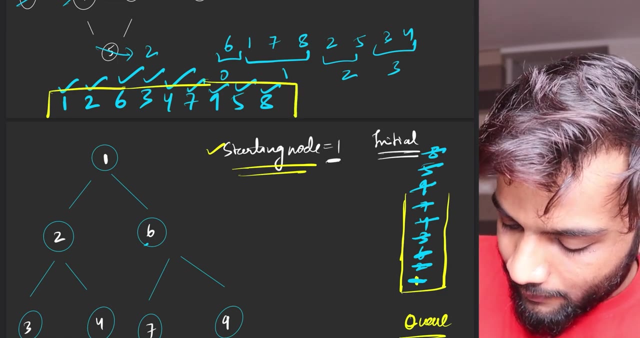 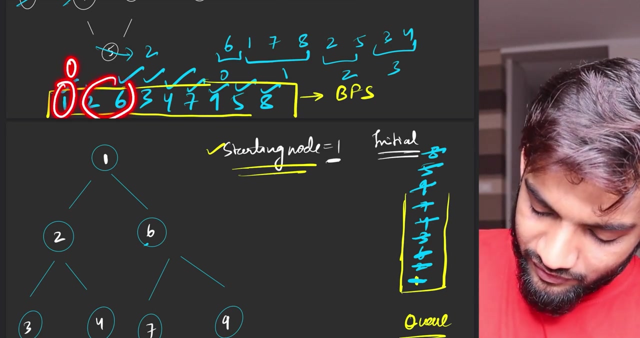 so no need to do anything. five is also done. next, take eight and for eight. if you see five and seven are already visited, no need to do anything. so this is also done. apparently, if you see, this is your bfs traversal. yes, this is your bfs traversal: zeroth level, first level, second level and the third level, if you carefully see. so we were. 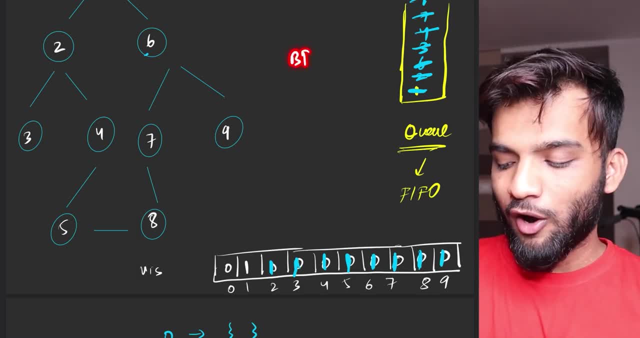 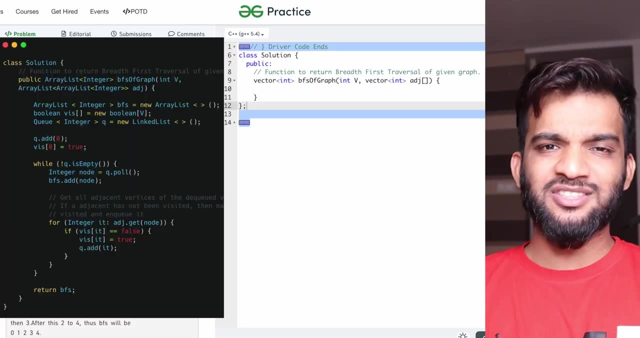 successfully able to print the bfs traversal of a particular graph. right now it's time that we check out the code. so i hope you have understood the entire explanation. now it's time to check out the c++ code and the java code, and we will see you in the next video. bye, bye. 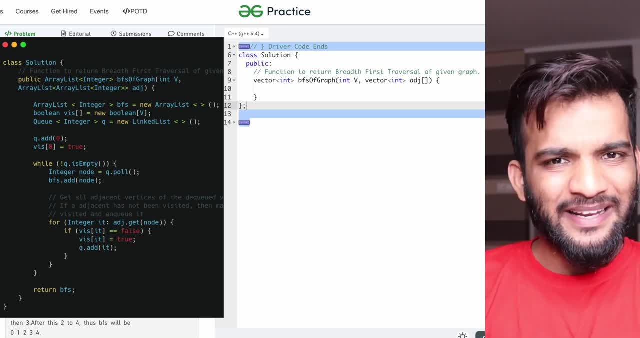 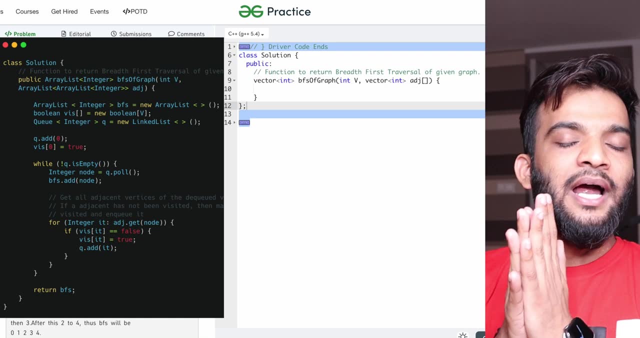 so what i'll do is i'll write the c++ code and i'll explain every step and the java code is on the left, so that you can just follow. for every corresponding c++ step, what will be the java code, and we are going to follow the same structure of code, so you'll not face a problem. so, generally, 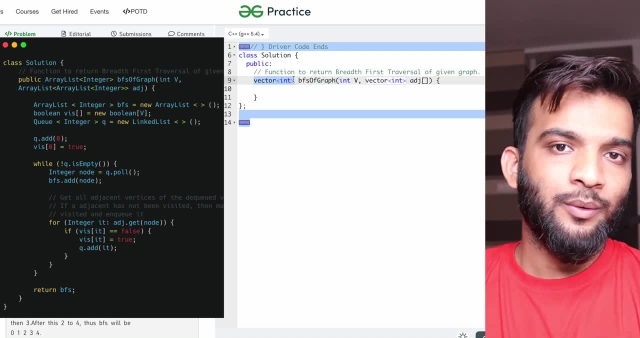 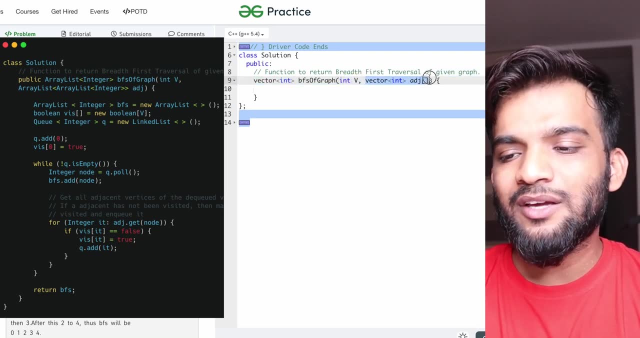 what will happen is you'll be given, uh, something like vector int where you have to store the bfs and return, and always you'll be given the number of nodes and you will be given the adjacency list. you don't need to create the adjacency list, they'll be giving you the adjacency. 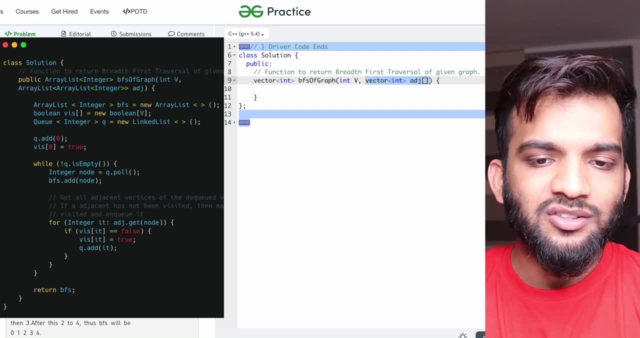 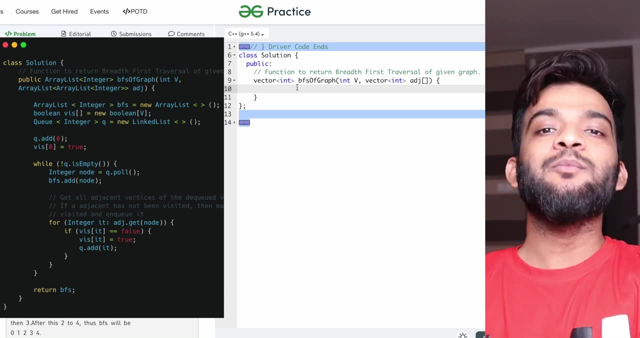 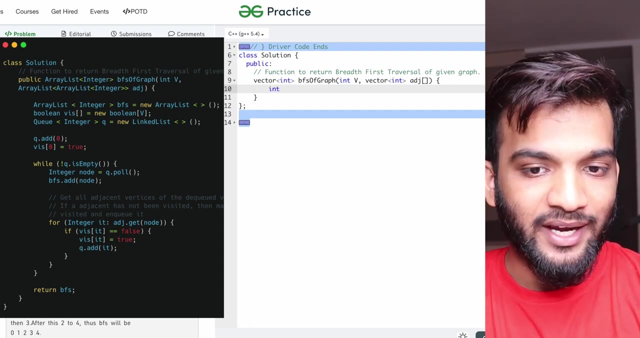 list in almost all the problems. now, this problem uh states: uh, a directed graph. but we will be coding this for an undirected graph, and then i'll tell you why the same code will work for directed graph as well. okay, so what is the initial step, if you remember? so first let's quickly check if this: 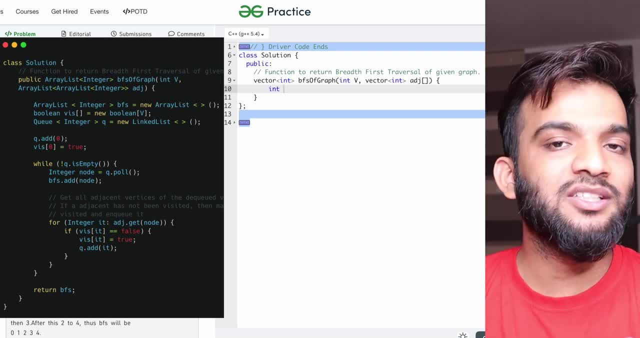 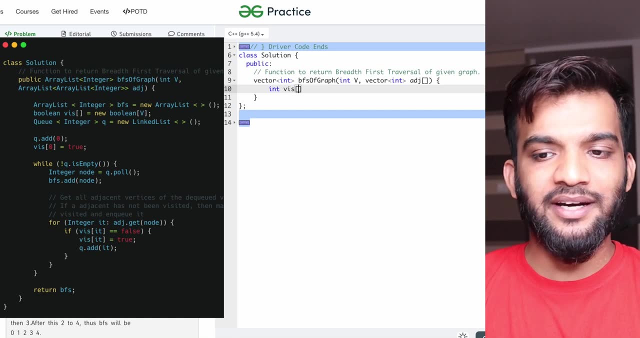 is a zero based indexing graph. so, if you see, it is a zero based indexing graph because the graph is starting from zero, right? so what you will do is you will just create the int visited array of n size and probably mark everything as this, and you know the initial configuration will be. 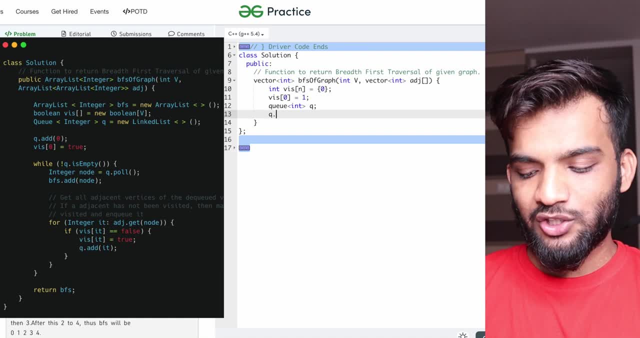 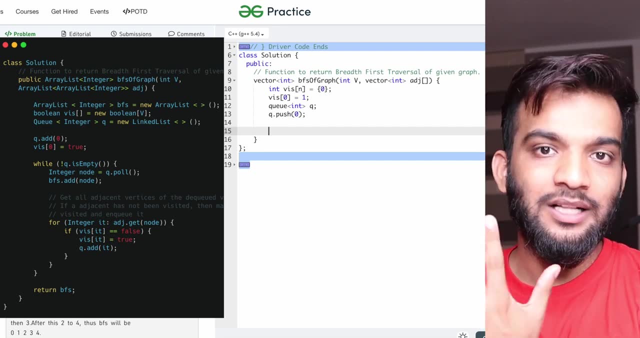 having zero and we will have a queue. okay, and in the queue, you know it will, it will be having the starting node done. now, what we did, we always took out everything from the queue till there was something in the queue. so can i say, always take out, like till it is having something, till it is. 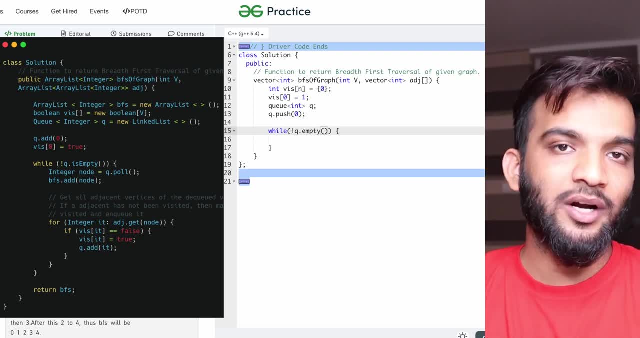 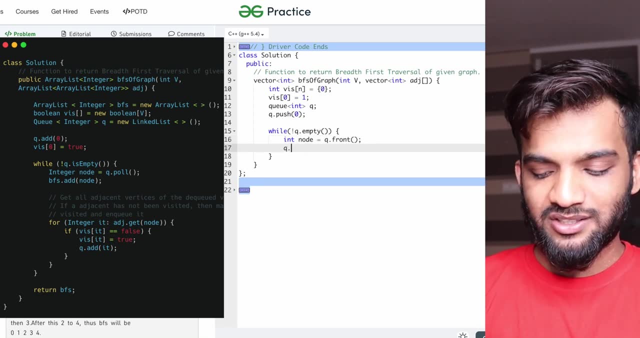 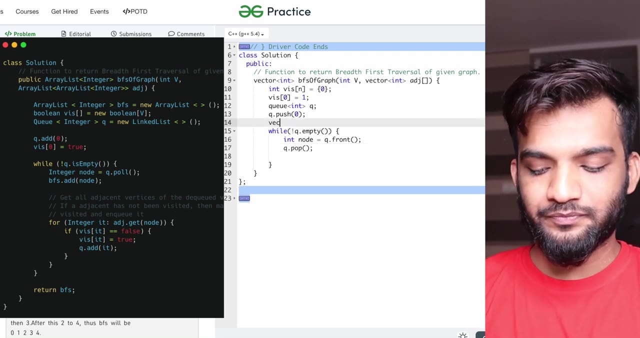 having something till the size is like still is not empty. just take it out and i can say: the node out like it will be qfront and we can just see qpop. so this will make sure you always get the node. and can i say, if i have to store the vfs, i probably can just, uh, do it over here and i can. 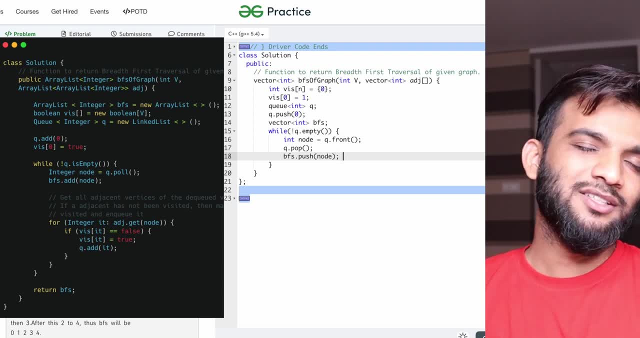 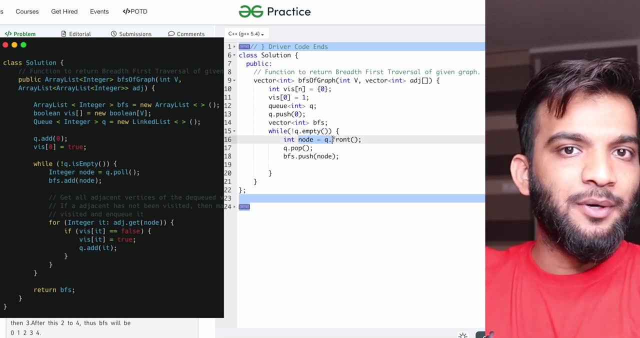 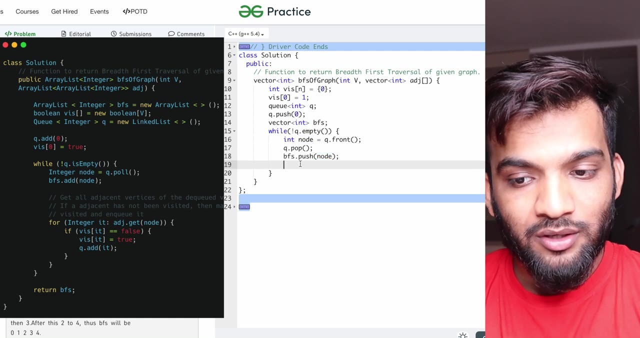 easily store, whichever node comes out. that's that. that is what gets into the bfs done. what is the next thing that we did? we always took out the node, if you remember, and we checked out its neighbor nodes, right? so who is storing the neighbor nodes? yes, the adjacency list. so for this node, can i see if i do auto of it of adjacency node. 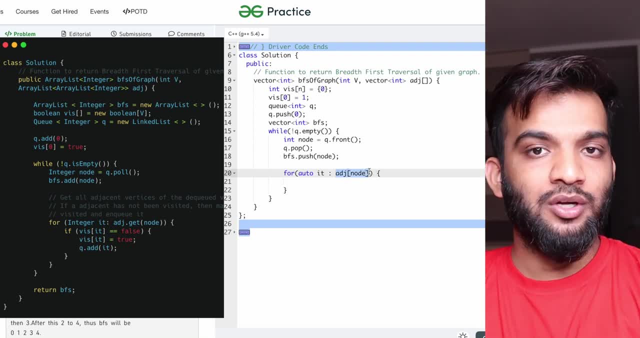 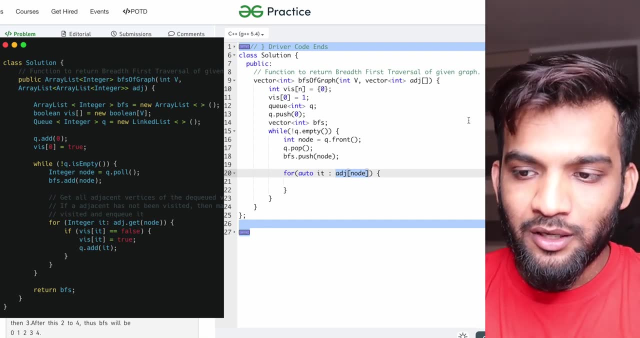 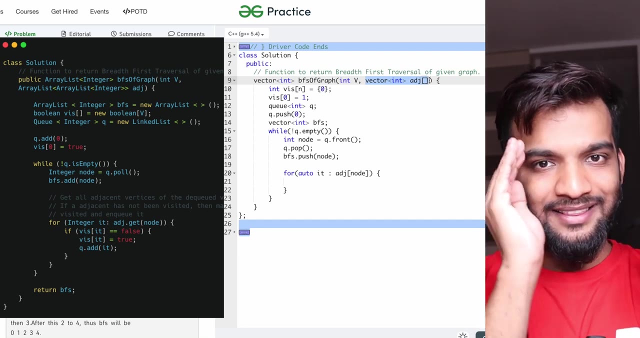 what does this mean? whenever i write adjacency node, i'm saying index node, that adjacency element will be a vector. if you remember the vector adjacency list, if you remove the list, if you say index, that index is storing a vector and that vector is storing all the neighbor elements. so 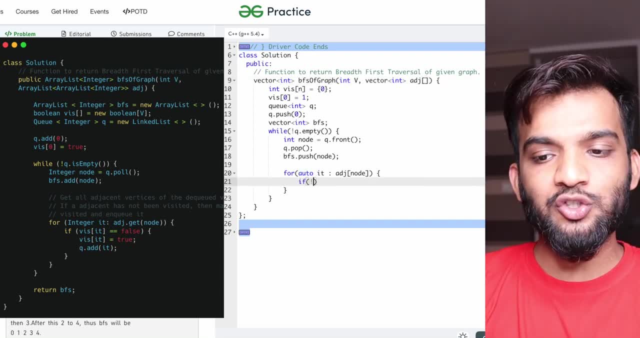 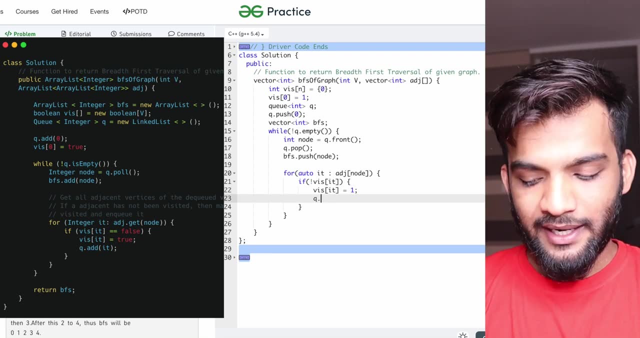 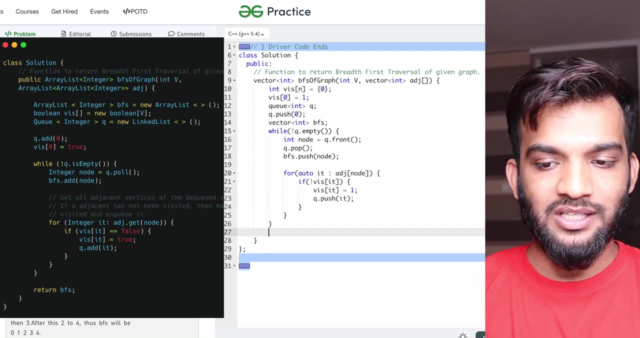 i iterate on them. so these are the neighbor elements. it you just need to check: have they been previously visited? if not, you say, okay, let me visit them. very simple, and let me put them into the queue as well so that in the next step, they can be taken into the pfs. once this is done, you 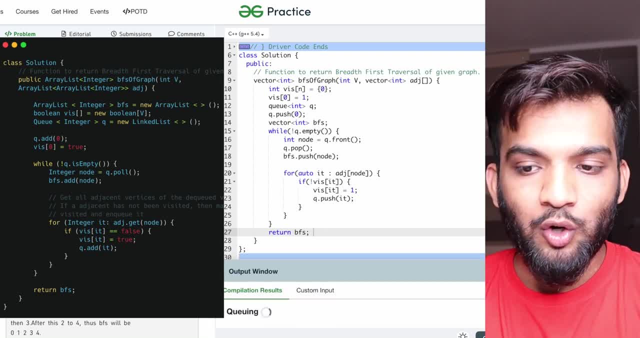 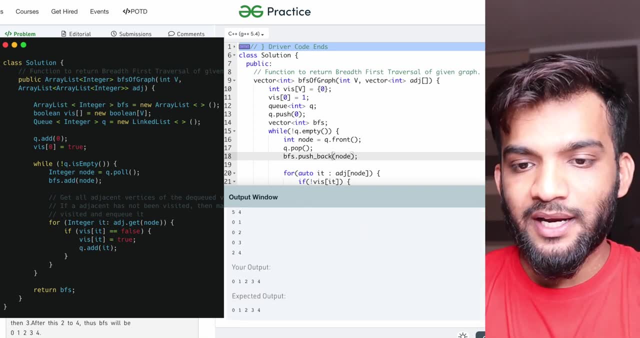 can say: this is my answer. once this is done, you can always say: this is my answer. okay, now let's quickly compile this and check, so if you see, uh, the compilation is successful, and let's quickly the code and check if it's working fine, and so it's time to understand the space complexity. 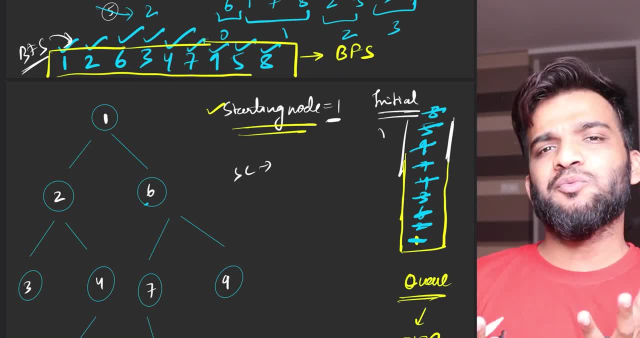 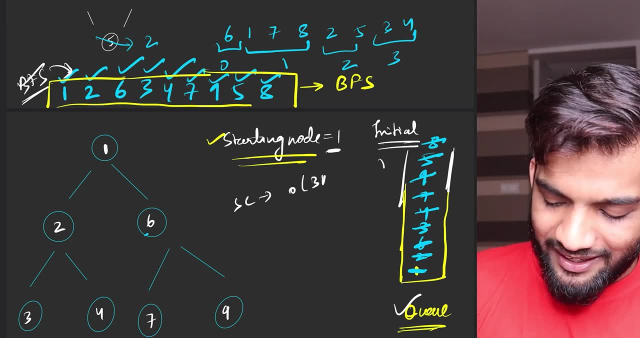 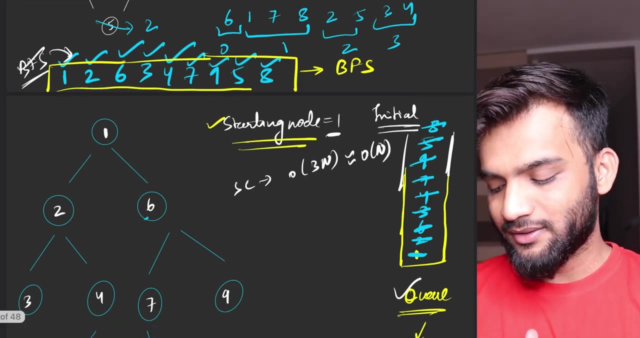 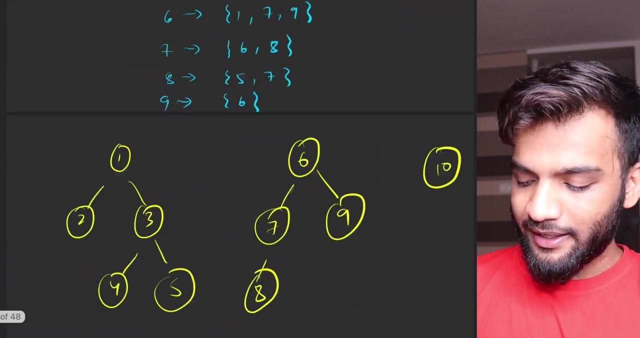 and the time complexity. space complexity is very simple: a queue, a visited node and a bfs list. so b go of 3n, which is almost equivalent to b go of n, and the adjacency list is given to you, so you can just omit this. and what about the time complexity? the time complexity is very simple. now, if i go and